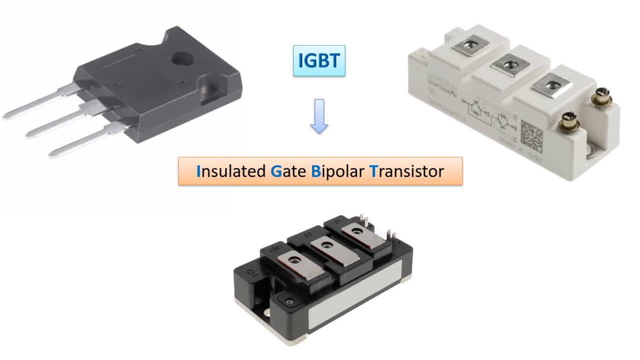 circuit element formed by the development of the best features of the MOSFET and BJT transistor. It appears in many areas used for switching purposes. IGBTs, which can act as triacs or transistors when needed, are used extensively. 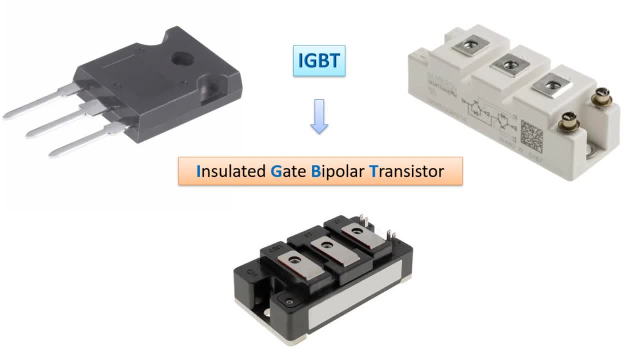 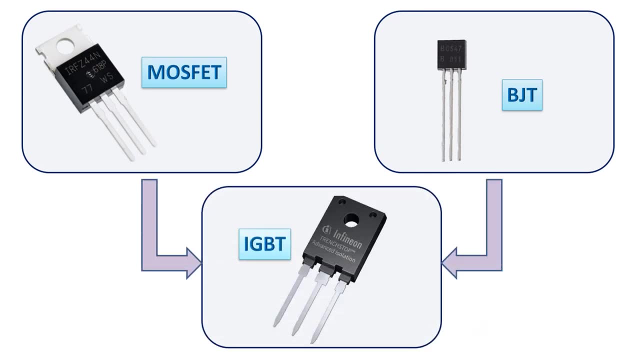 especially in UPSs that require high switching speed. The IGBT is the combination of BJT and MOSFET. Its name also implies the fusion between them. Insulated gate refers to the input part of MOSFET having very high input impedance. 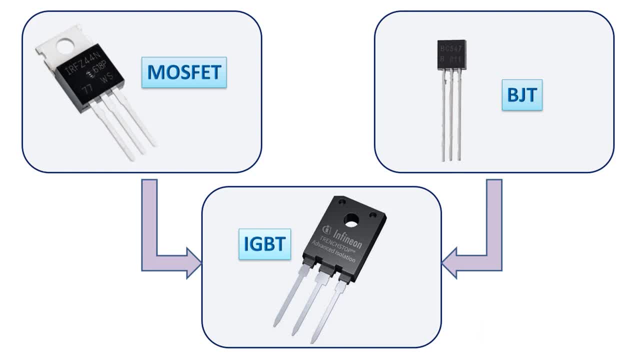 It does not draw any current between it and the MOSFET, any input current. rather, it operates on the voltage at its gate terminal. Bipolar refers to the output part of the BJT having bipolar nature, where the current flow is due to both. 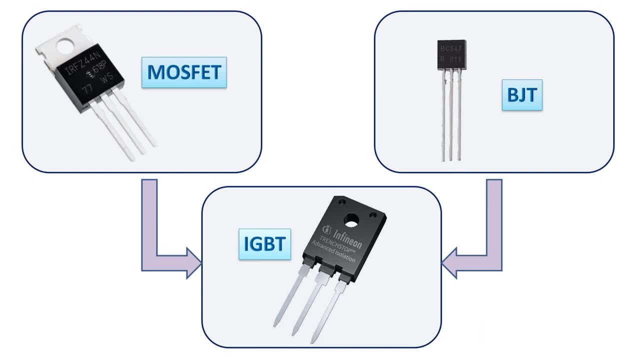 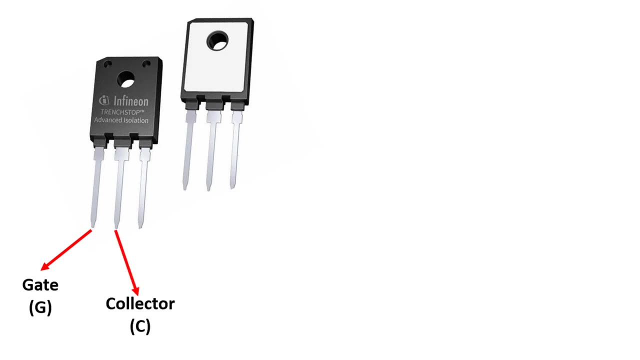 types of charge carriers. It allows it to handle very large currents and voltages using small voltage signals. This hybrid combination makes the IGBT a voltage-controlled device. IGBTs have three pins. One of them is the gate, the other is the collector. 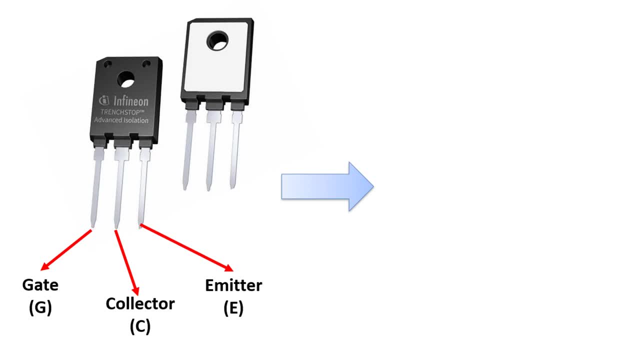 and the last one is the emitter. The abbreviations G, C and E are used for these. Their locations may not always be like this. Pin locations may change according to the type Their symbols are. as you see on the right, These two symbols are also used. 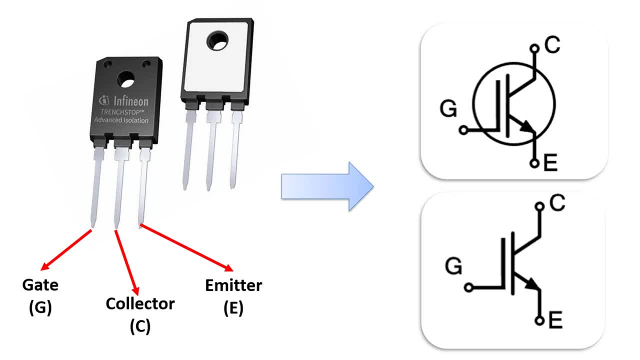 You may encounter symbol drawings similar to these that differ slightly, as can be understood from the pin names. we can understand that it shows both MOSFET and BJT transistor features. If you remember, the gate pin is located in the MOSFET. 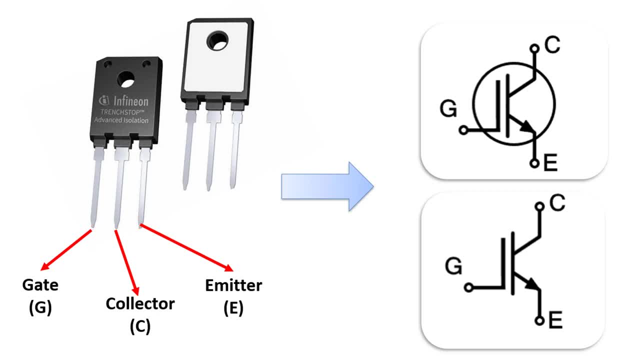 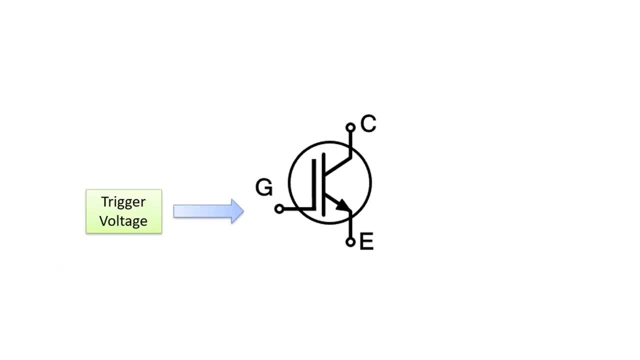 while the collector and emitter pins are located in the BJT transistor, The working logic is similar to the working principle of the same MOSFET. With the trigger voltage applied to the gate pin, a large current between the collector-emitter is controlled. In other words, as in the same MOSFET, current control. 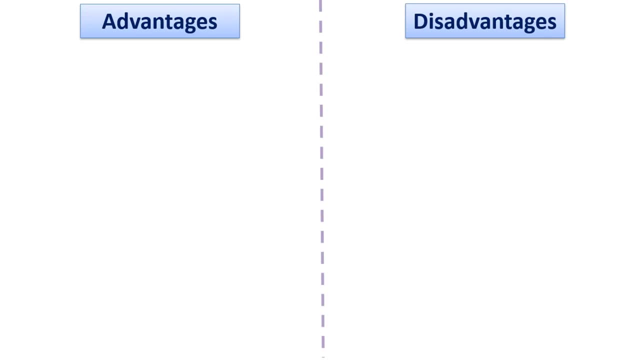 is provided with voltage. Now let's look at the advantages and disadvantages of IGBTs over BJT and MOSFET transistors. As a whole, IGBT has the advantages of both BJT and MOSFET. If we start with the advantages,